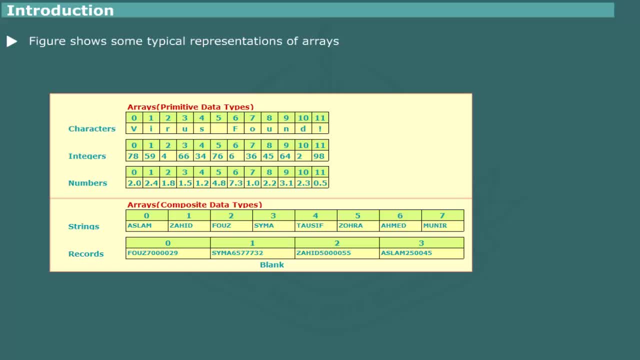 Notice that in the first example, all of strings are of same length, Consisting of six characters. If there are fewer alphabets, the extra places are padded with spaces shown as Bs. The second example represents an array of employee record. 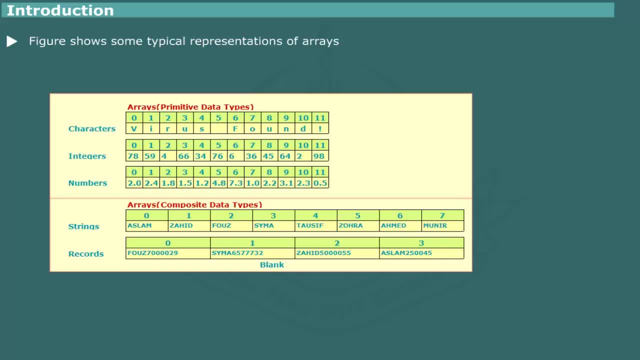 In order to preserve the homogeneity property, each record should have the same size and same composition of fields. For example, the name field cannot be the same as the name field. The name field cannot be 20 characters long in one record and of 30 characters in another record. 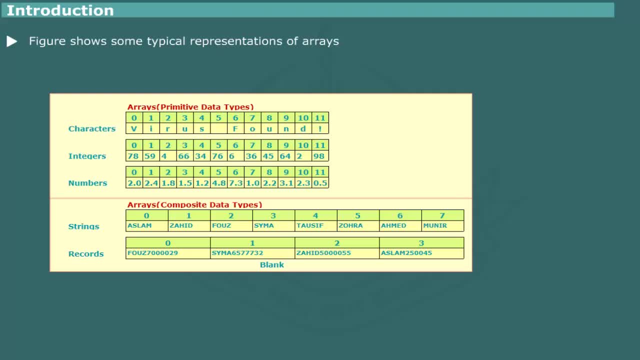 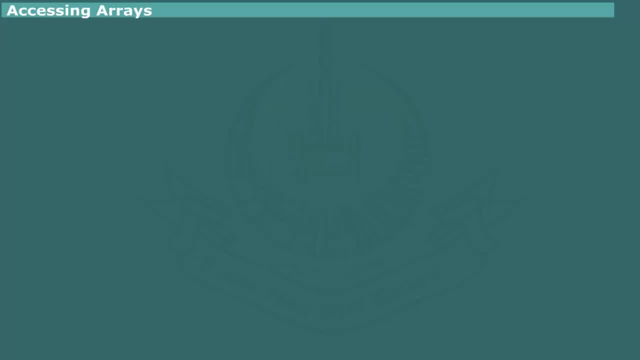 Likewise, the salary field must be either integer type or floating type in all of the elements Accessing array. Each array structure is identified by a unique name. The position of each element within the array is identified by a variable called index. The range of index is referred to as index set. 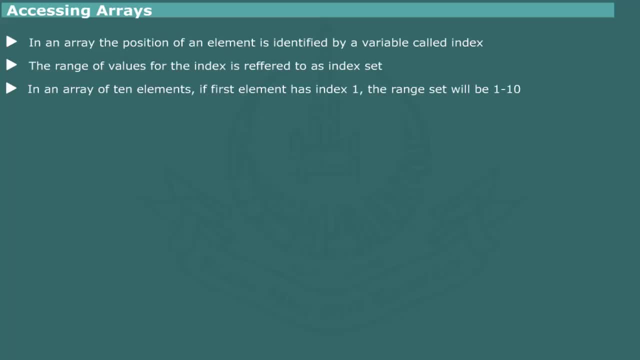 For example, an array consisting of 10 elements would have an index set of integers varying from 1 to 10.. Sometimes, the first element of array is counted as the zeroth element. In this case, the index set would have range from 0 to 9.. 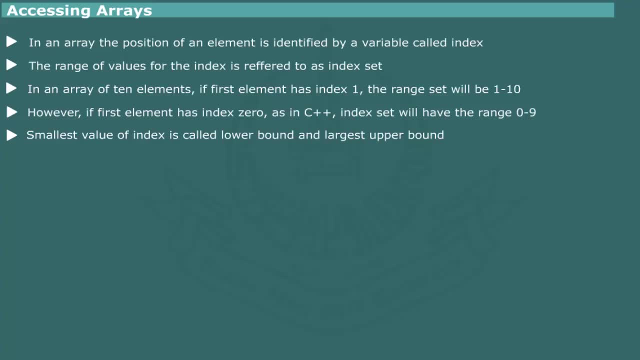 The smallest value of index is called lower bound and the largest value is called upper bound. Thus, the size of an array is given by the relation. The individual elements of an array are identified by the array name and array index. For this purpose, different notations are used. 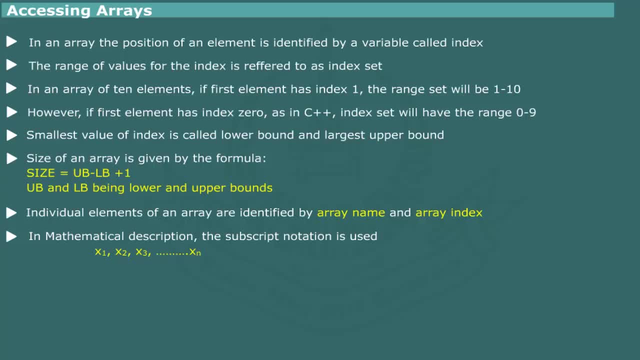 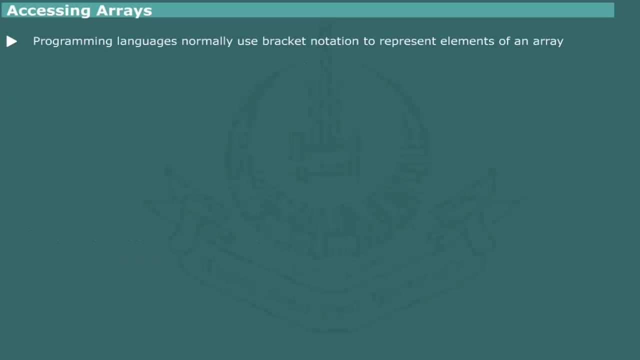 In the mathematical description of an array, the subscript notation is used. For example, the elements of array x consisting of n elements are denoted by the sequence. The programming languages, however, use bracket notation for array elements. The elements are defined by the array name, followed by either parentheses or a pair of square brackets that enclose the index value. 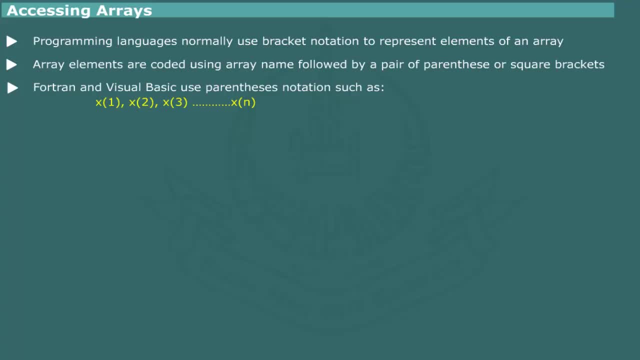 Porton and Visual Basic use the same notation. Porton and Visual Basic use parenthesis notations such as c, c++ and java use square bracket notation. Thus, elements of array x are denoted by. Sometimes, index is also referred to as subscript and index set as subscript variable. 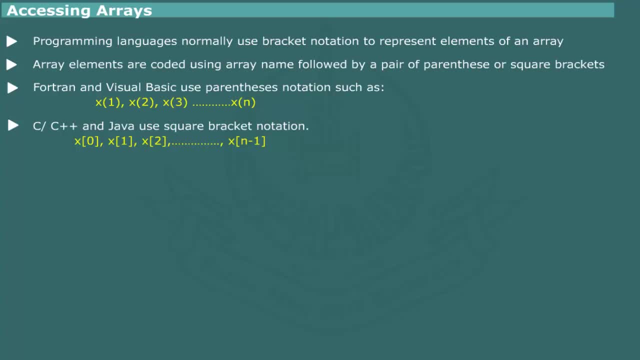 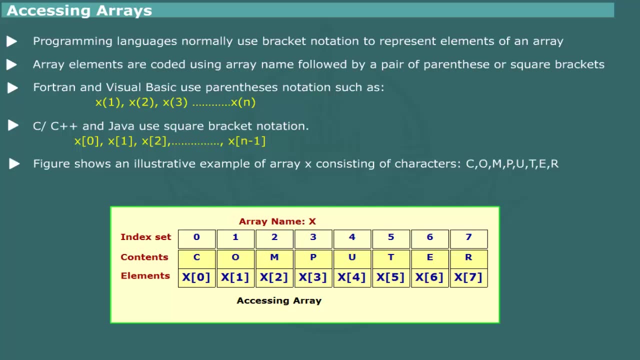 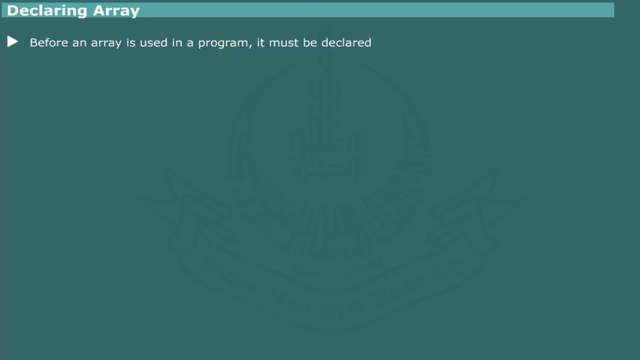 The contents of an array are often pictured using the name and index value. Figure shows an illustrative example of array x consisting of characters c, o, m, u, t, e and r. Declaring Array. Before an array structure is used in a program, it must be formally declared. 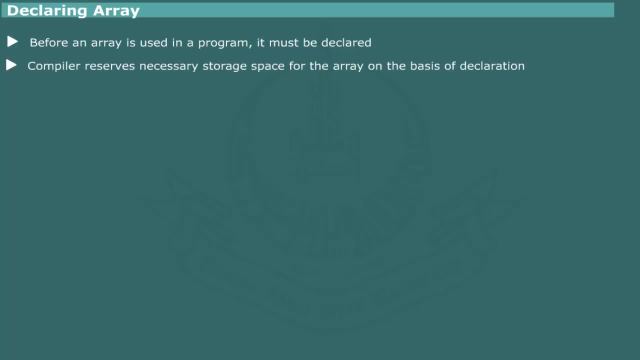 This is required by the compiler in order to reserve necessary storage space. The rules for array declaration differ with programming languages. In general, the declaration specifies array name, size and data type. In c, c++, for example, this declaration means that the array x would consist of a maximum 100 data elements of integer type. 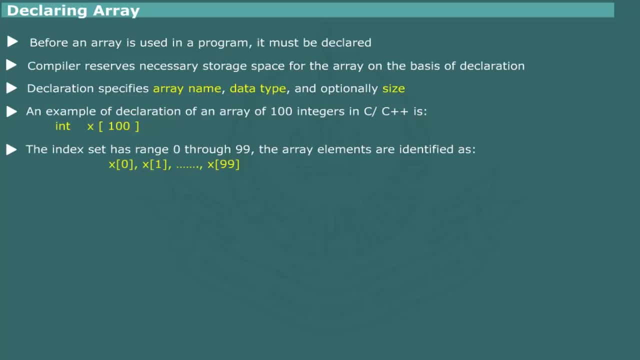 Further, it is implicitly implied that the index set will have the range of 0 to 99. In other words, the array elements will be denoted by. In subsequent discussion we will follow the c c++ notation and rules for declaring arrays. 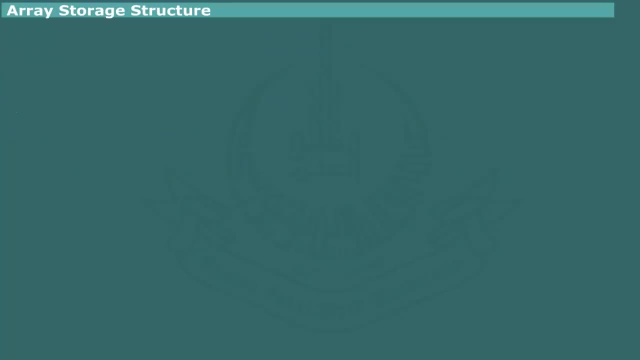 Array Storage Structure. Storage structure represents the arrangement of data elements in the memory of a computer. Array Storage Structure represents the arrangement of data elements in the memory of a computer memory of a computer. an array is always stored in contiguous memory locations. the number of storage cells allocated to each element depends on the data types. 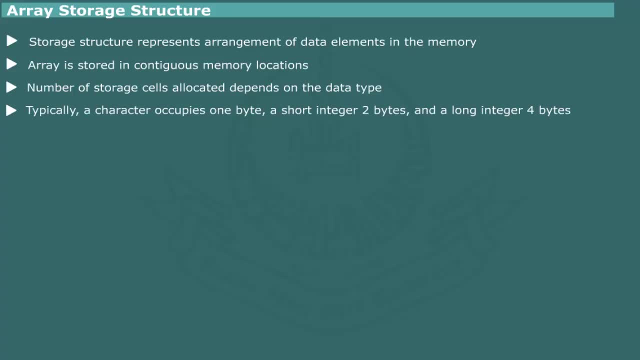 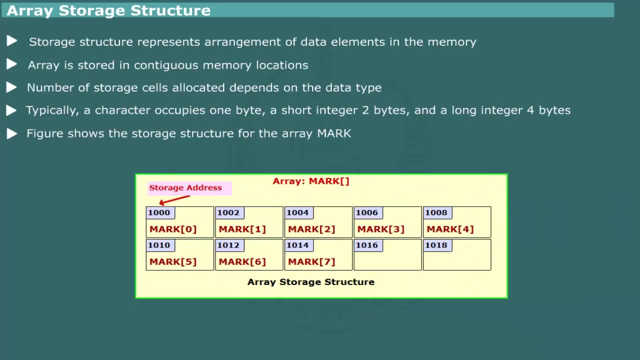 typically a character occupies one byte, a short integer 2 bytes and long integer 4 bytes. figure shows the storage structure for an array mark consisting of short integers in this storage map. the first element is stored at location 1000, second element at location 1002. 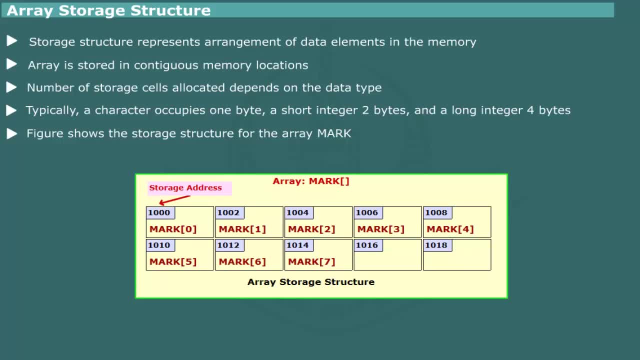 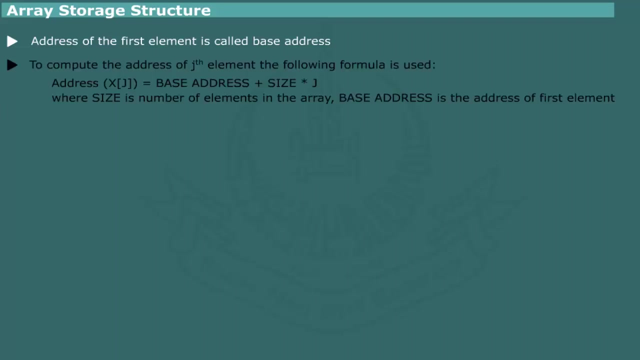 and so forth. the numbers 1000, 1002, up to 1014 are referred to as storage addresses. the address of the first element is called base address. in this example, the base address of array mark is 1000. by knowing the base address we can easily compute the addresses of other elements by using the general formula. 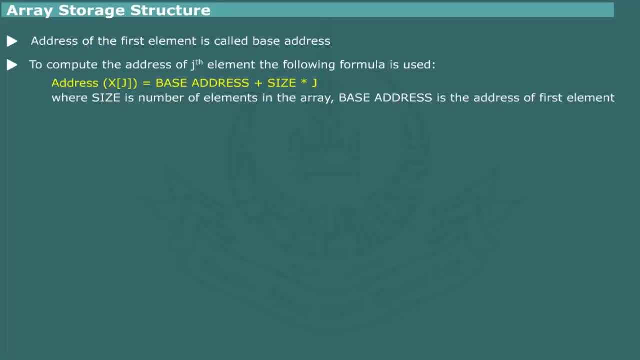 where address xj means storage address of the element xj, j being the index, and size is the address of the first element, x0, and size is the number of bytes allocated to an element. thus, using the index, we can easily compute the address and access the element without the need for searching other elements in the array. 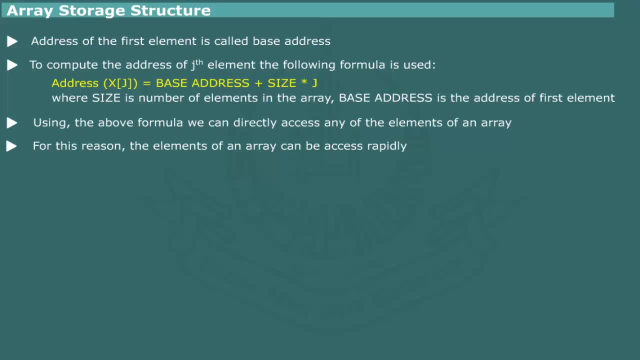 for this reason, the elements of an array are said to have direct access. further, we do not have to keep track of elements in the array. we only have to keep track of the base addresses of all array elements. only the base address is required to process other elements in the array. 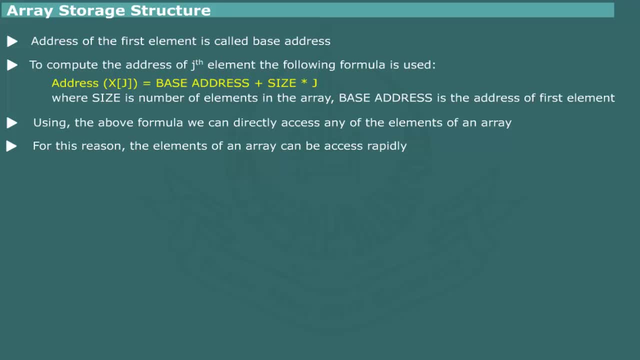 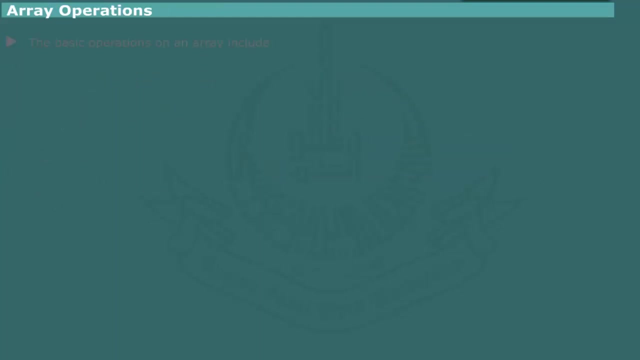 it would follow that storage structure for an array is quite efficient. it has, however, the drawback that memory allocated to an array is not released until the program execution is finished. array operations. the basic operations on an array include retrieving an element, adding a new element to array, deleting an existing element. 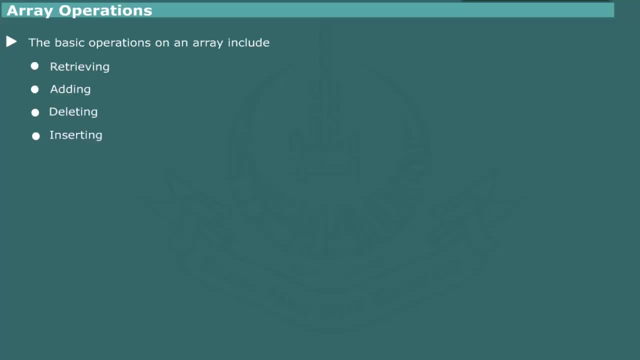 and inserting a new element. in addition, we can perform some auxiliary operation to determine the current status of the array or obtain some information about a specific element. these operations might include the following: checking if array is valid. full checking if array is empty. getting index of a specified element. and. 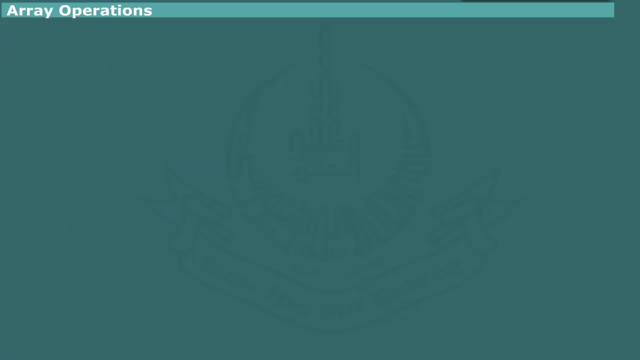 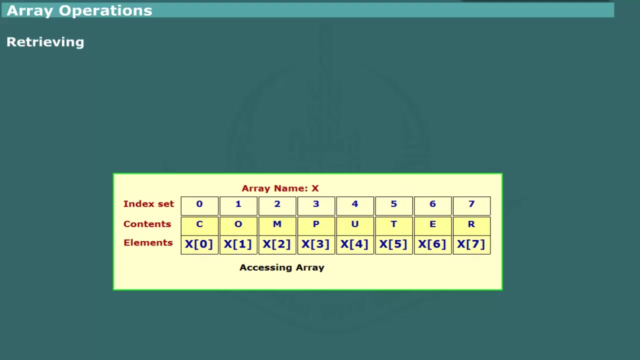 traversing to process array elements. retrieving. retrieving an element is the most common operation. it is also called accessing. to retrieve an element, we need to know the index value. for example, mark J would access the date element of array mark. as noted before, the computer can directly retrieve an element without 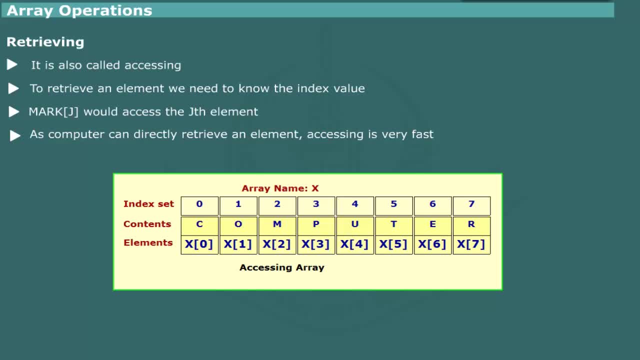 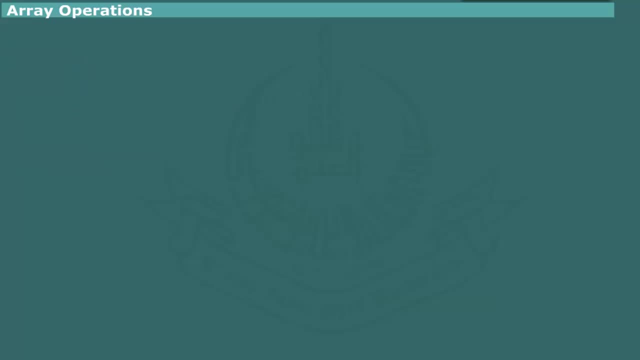 examining other elements in array. thus accessing operation is very fast. further, since the access is independent of the number of elements in the array, access operation has a time efficiency Oh one adding. the add operation places a new element in the array in a position specified by the index. it is also called assignment operation. thus, if we want to, 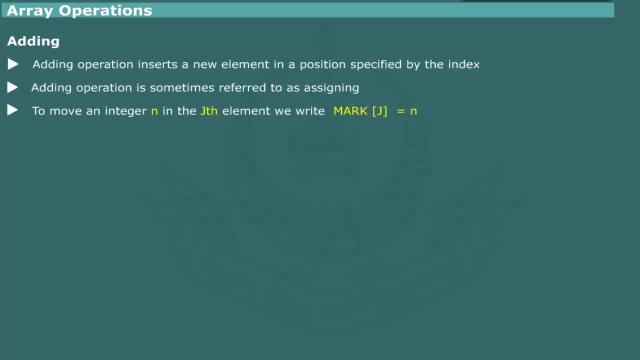 move an integer n in the date element of array mark, we simply write: mark J is equal to n. if the array already contains some element in the specified position, it is replaced by the new element. The add operation has time efficiency O1.. Deleting The delete operation removes an existing element from the array In order to delete an. 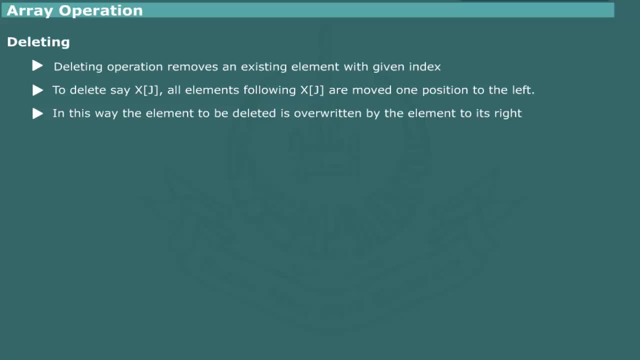 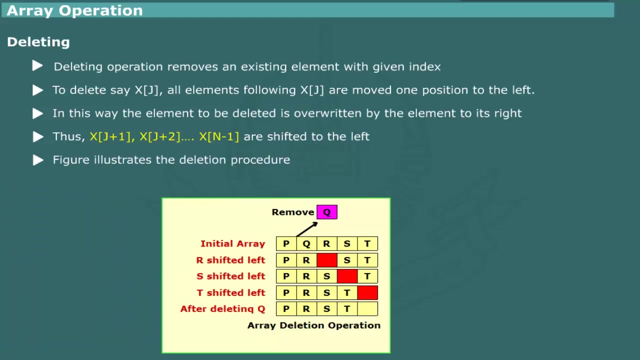 element, say xj, we simply move all elements after xj one position to the left. In other words, elements xj plus one, xj plus two up to xn minus one, where n is the array size, are shifted to the left. Let us consider the process of deletion of an array element. 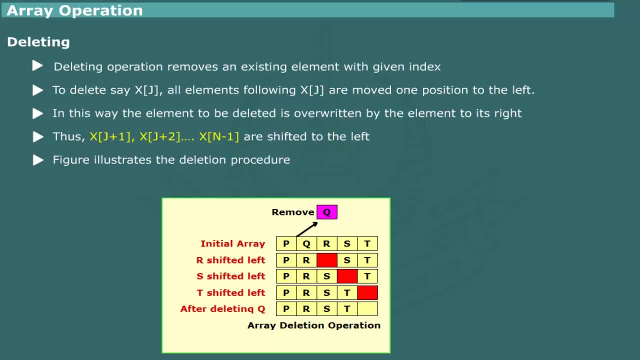 The array shown initially contains letters p, q, r, s and t. In order to delete q, the element r, s and t that follow q are shifted one position to the left. Notice that the deletion of q does not release any memory space occupied by the array. The elements r, s and t are simply reorganized. 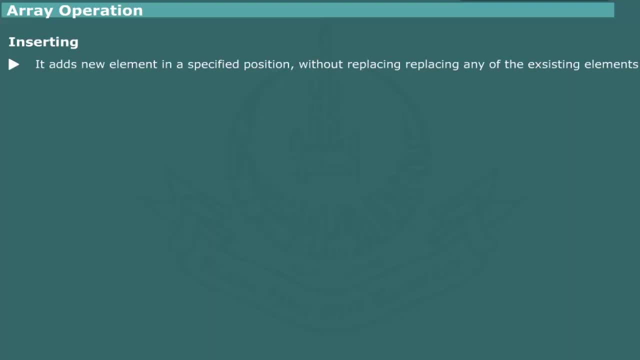 Inserting The insertion operation adds a new element to the array in a specified position, without replacing any of the existing elements. The position of the elements may be specified in terms of index value or relative to an existing element. The new element might, for example, be placed before a given element In order to insert. 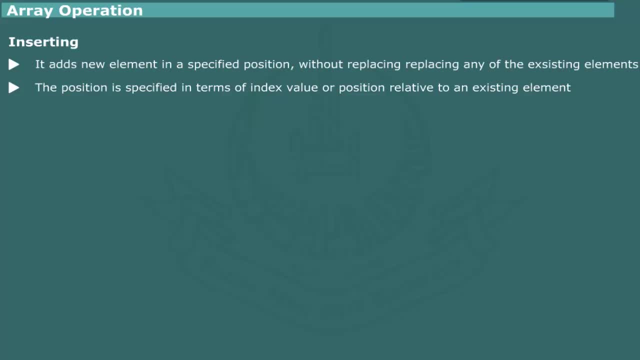 a new element in specified location. all elements to the right of element are being moved one place to create a room for the new element. For example, if a new element is to be inserted, it is placed before an element. For example, if I move a element to the outside, it will move to the inside and it will move. 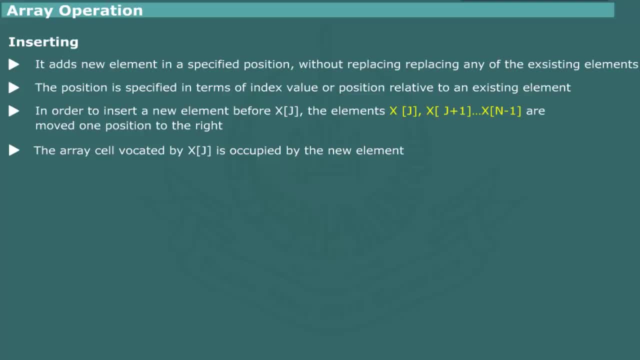 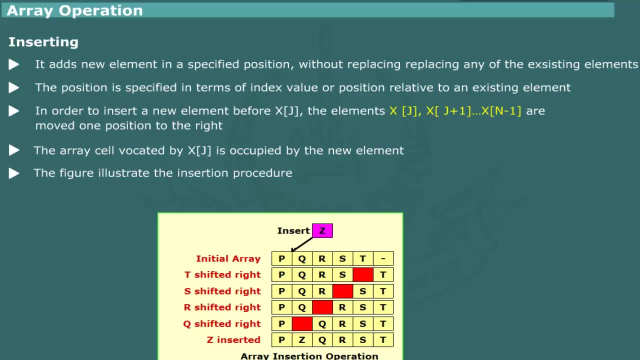 to the outside. So in order to insert a new element, I need to insert a function in the array that contains the x, j, xj, xj plus 1 up to xn minus 1.. This is to be moved one position to the right. 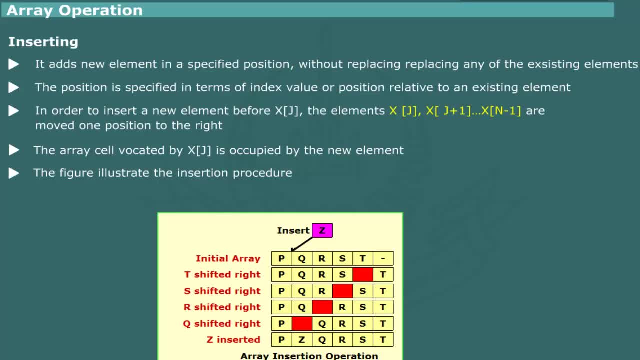 Let us consider an example to demonstrate the insertion process. The array shown contains letters p, q, r, s, t initially. In order to insert an element z before the insertion operation, the array is adjusted to x, k and z. 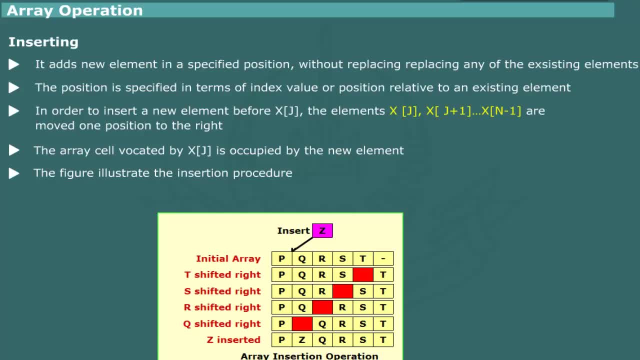 In order to insert an element to the left of element, the array is divided and the element y, q, x, x and t are moved one position to the right. For the element r. the elements r, s and t that occur after r are moved one position to the right. 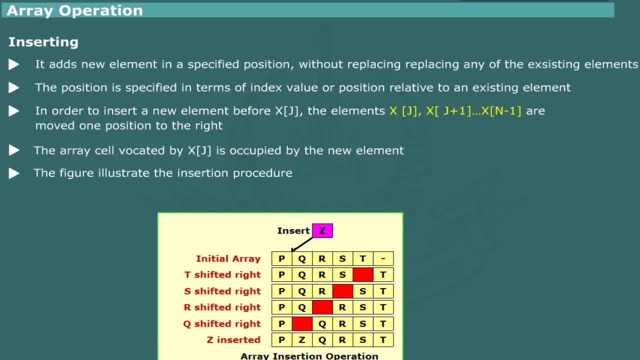 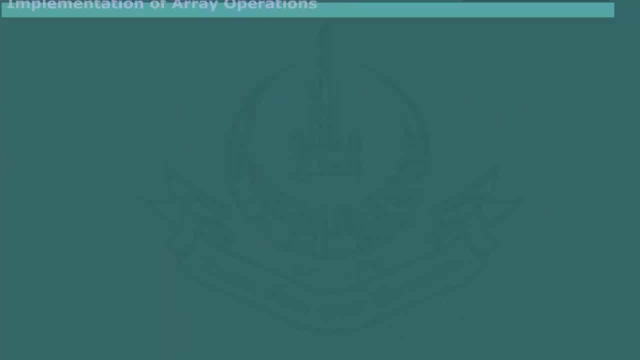 The space created due to shifting of r and other elements is filled with the new element z. Observe that after insertion of z, the array size increases by 1.. Also note that no additional memory space is allocated to accommodate the new element. Rather, the elements are simply rearranged within the memory block initially reserved for the array. 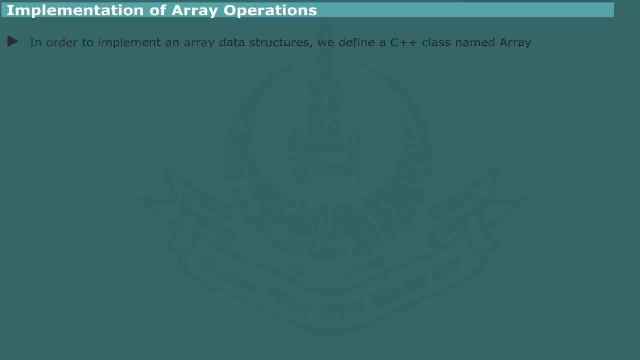 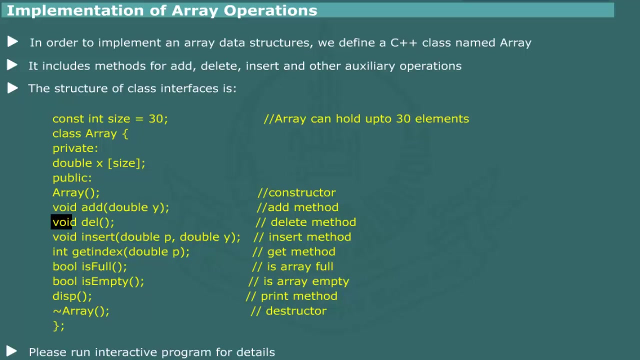 Implementation of array operations. In order to implement the basic operations on array, we define a C++ class named array, which includes add, delete, insert and other operations. The structure of class interfaces is shown. Add appends a new element. Delete removes an existing element.